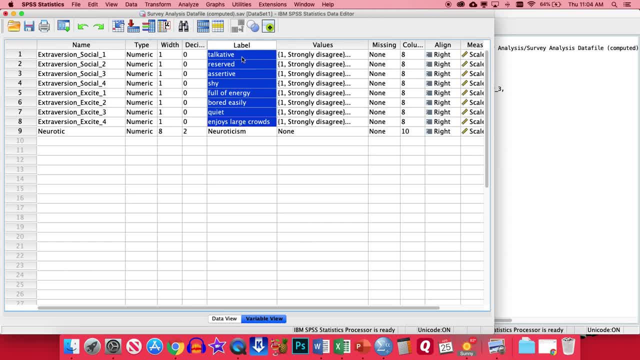 basically pointed in the wrong direction, where a high score actually means that someone's introverted- So for example, reserved- is one of those reverse scored items, And so to mark that down, we're just going to add a- what do you call it, that little line thing? and then the 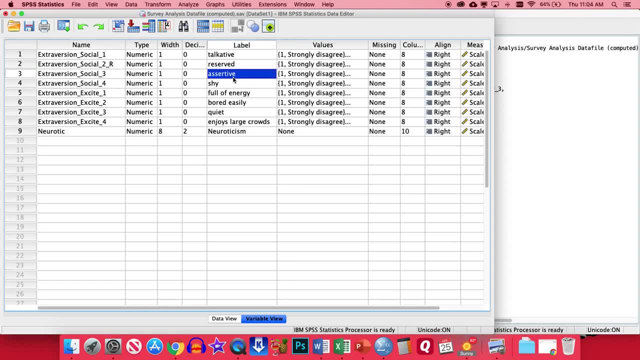 uppercase R, meaning that's reverse scored. Now, being assertive, that's being extroverted, so that's totally fine. But being shy, we're also going to add an R to that as well. Being full of energy, that's being extroverted. But being bored easily, oh, actually, that is actually also being extroverted as well. it's a high need for excitement. 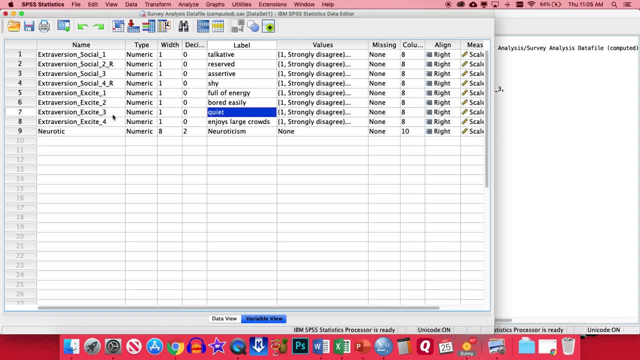 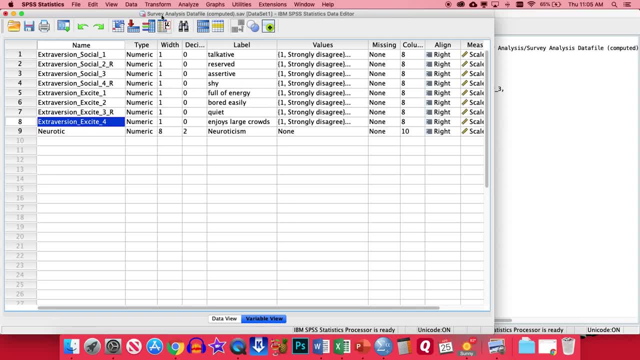 So all we're doing is marking down in the name which ones need to be reverse scored. These are the items that we need to flip the scale on and so on. So to do that reverse scoring, we're going to go up to transform recode to different. 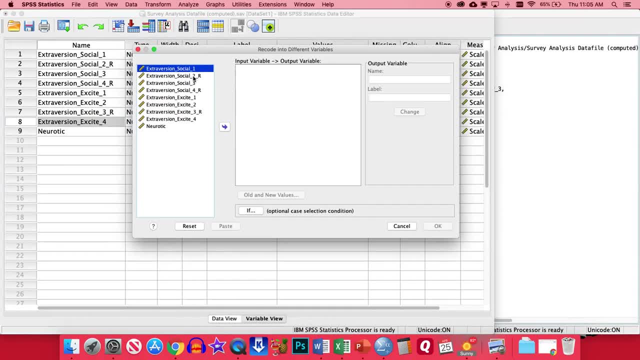 variables, And since we've already located the ones that need to be reverse scored, it's really easy to pop those then into the numeric variable box And basically we're going to give them the same name as they have before, just minus that underscore R. So this one will be extraversion. 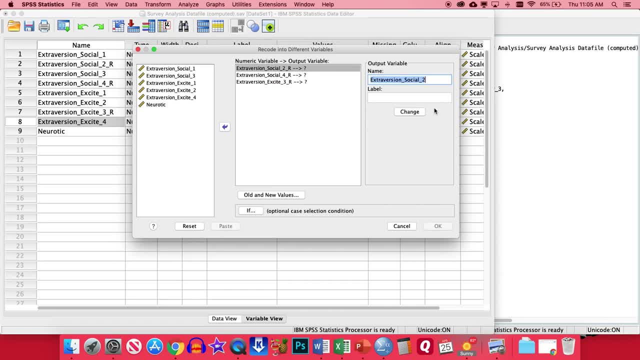 underscore social, underscore two, And I'll just sort of copy that and make it a little bit easier to create these same names. This one belongs to the excite factor, So I'll change this to excite and it's the third item. So after you've given them the same name, just minus the underscore R. 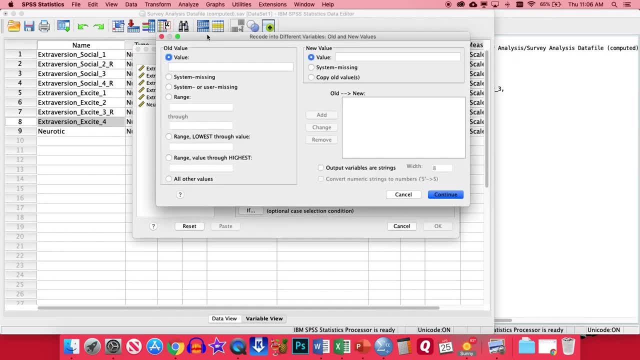 then we're going to flip the scale by going to old and new values, And here we're going to take the old value and turn it into its opposite. So if it's a one on the one to five scale, the opposite of that on the scale would be a five. Similarly, if it's a two, the opposite of that. 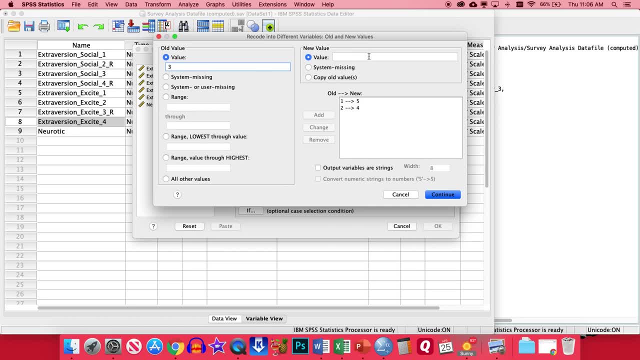 scale would be a four, And if it's a three, since that's right in the middle of the scale, it'll remain a three, But then we'll go backwards from there. So a four will become a two, and then a five will become a. 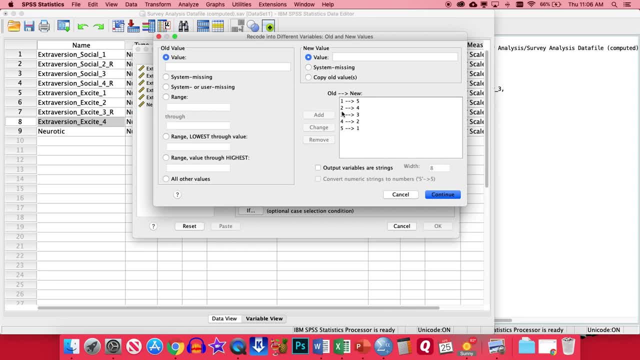 one. A nice way to check to make sure you haven't missed anything is if you go in columns it should count one, two, three, four, five, five, four, three, two, one, And if this was a one to seven. 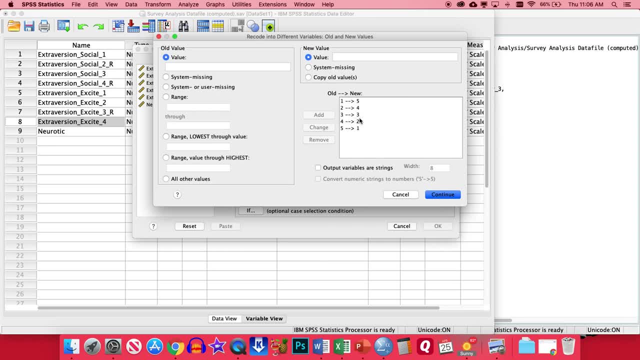 scale then it would be one, two, three, four, five, six, seven and seven, six, five, four, three, two, one. So it just has to include all of the types of items you can have in the scale. 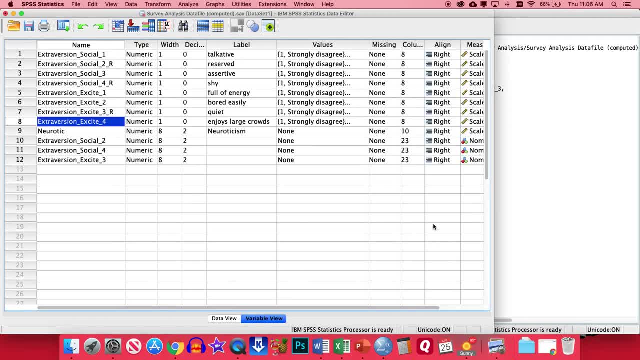 So that looks good, So we'll click on that, And then we're going to go to the next item and we're going to, So we'll click continue and okay, And basically that'll put our items right here. One thing I like: 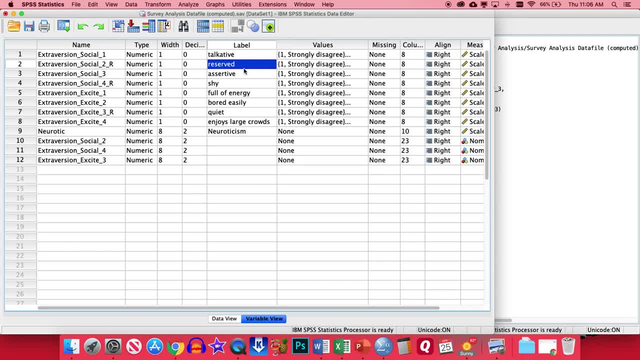 to do too is just copy the labels from the original items. So number two on the social scale would be reserved. So we copy that one in there. Four is shy, And then the third. one of the excite scale is quiet. That way we remember what these items originally referred to. But also now we have 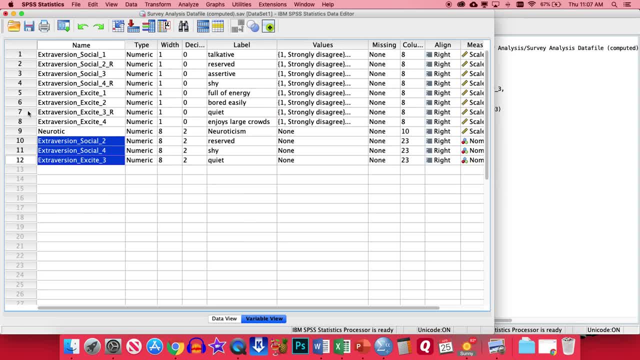 them pointed in the right direction. From this point on, actually, we won't end up using any of the items that are pointed in the wrong direction. We'll always use the ones that we've just created. So first thing we want to do is to figure out if these items are in fact reliable. So one thing we 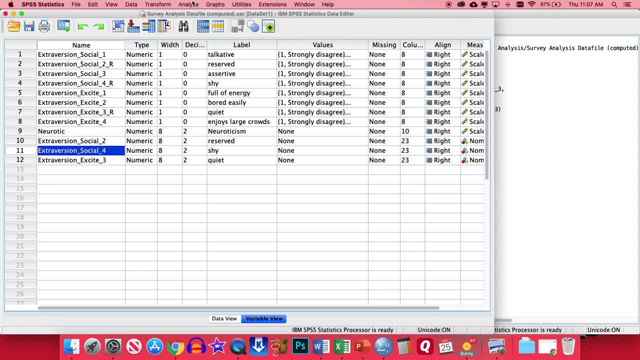 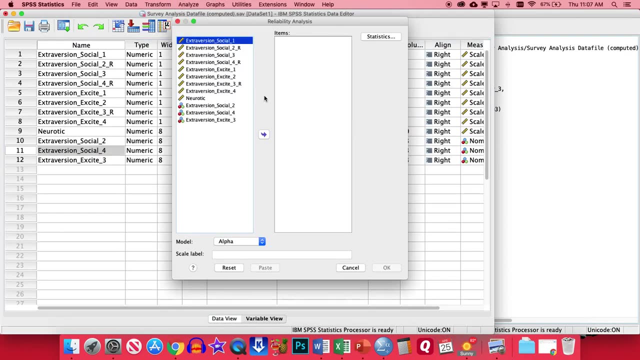 can do is a Chromebox alpha. That's a good way to test to see if there's inter item reliability or consistency. Basically means, are all the items measuring the same thing? So to do a Chromebox alpha, we're going to go to analyze scale reliability analysis. Now we're going to look at the social item. 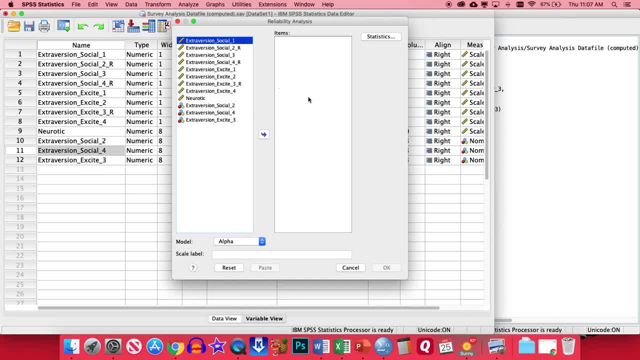 separately from the excite items, since they are part of two different factors. So for this one I'm going to put in all the social items. will put in Social 1. We're going to skip this one, that incident underscore r. We'll pop in social to the one we made right here. Go back up Pick. 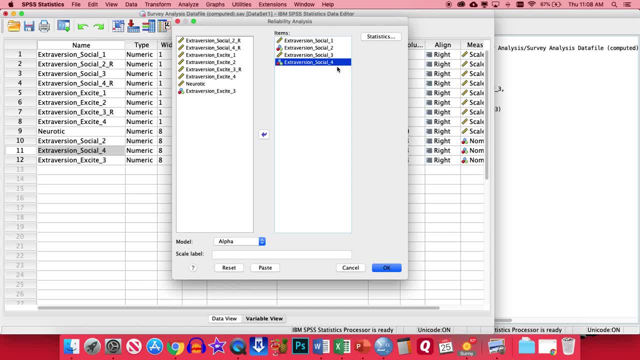 up social three, And then again we're gonna get social for, because that's the version that's pointing in the correct direction. So after you've done that, that's all you need to do. Just put in the items for the whole scale and then click okay. Basically, what a Chromebox alpha looks at is the: 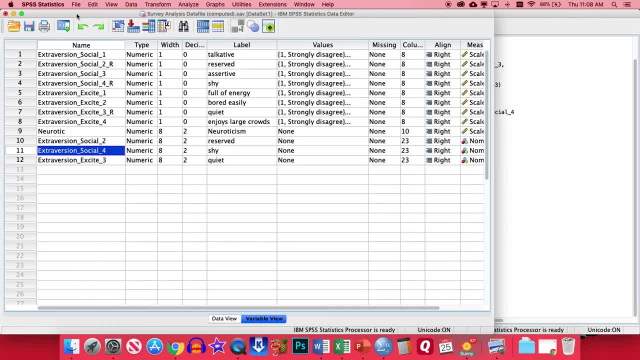 others page level of correlation between all the items. So if someone's strongly agreeing that they're talkative, they should also probably strongly agree that they're assertive and strongly disagree that they're reserved or shy. That would mean that all of them are pointed in the right direction. 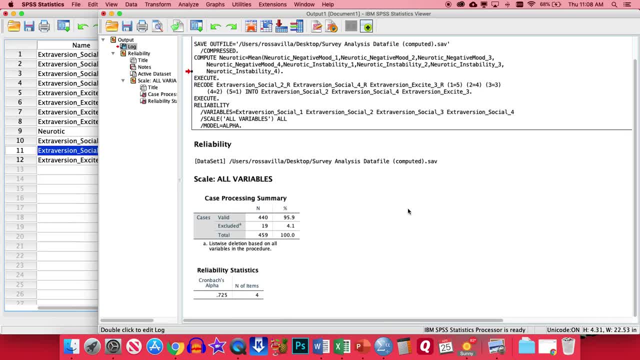 and measuring the same thing, And what we want to see is an alpha score that's at least a 0.7 or higher, And in fact, that's what we have here. So, if you look at the alpha score, Chromebox Alpha. 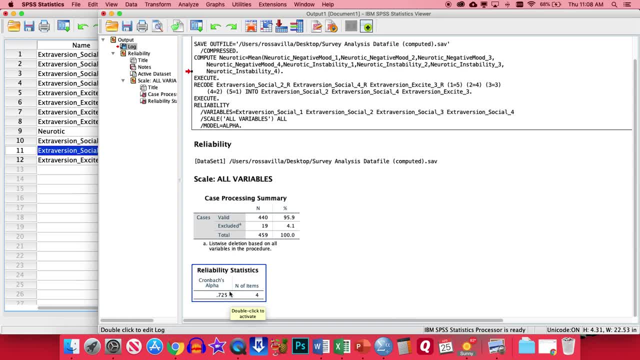 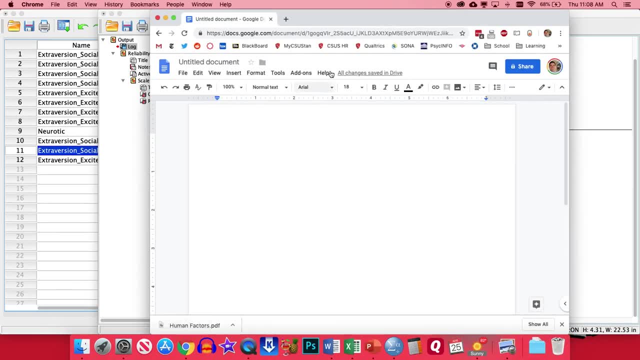 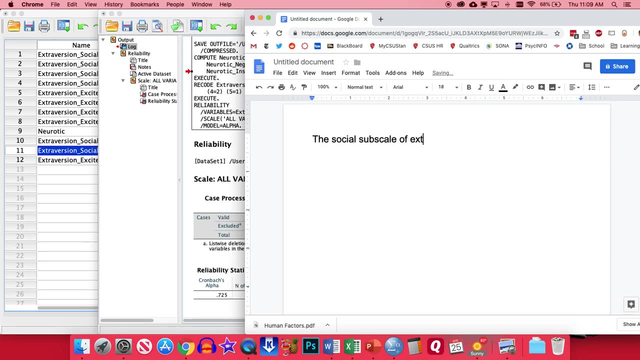 we have a 0.725.. So that actually means that we have good levels of inter-item reliability with that scale. So to write up something like this, I'm just going to open up a Word document here. I would just write something like the social subscale of extraversion. 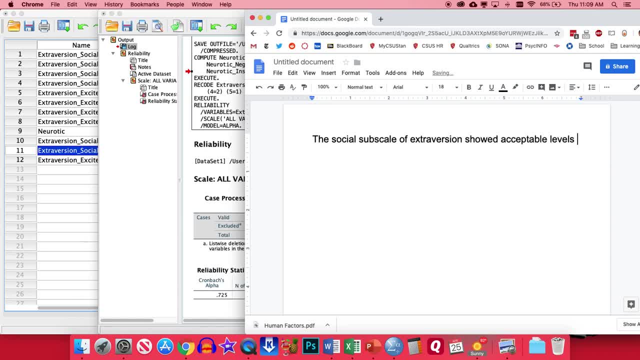 showed acceptable levels of reliability. And then I can put in the alpha score by just putting in an, A lowercase a for alpha and then putting in this number right here We're going to round it to the 100th place, So it'll be 0.73.. 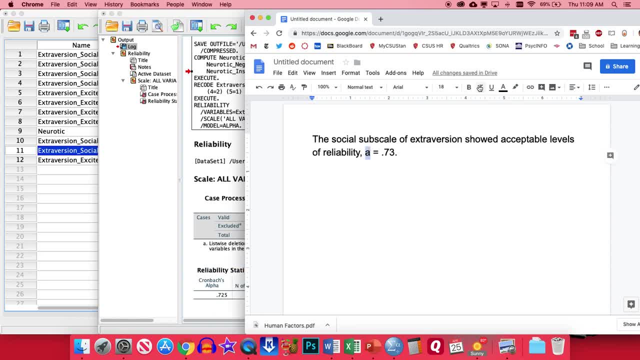 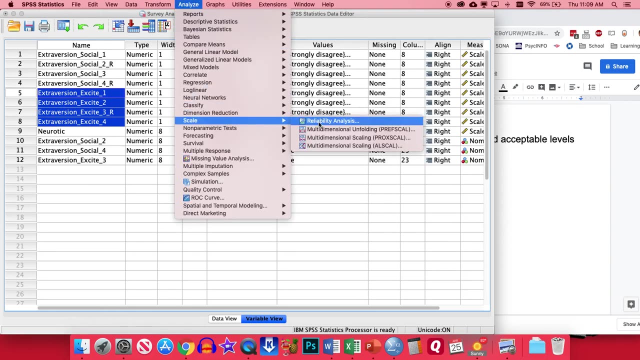 And then if we italicize the A there, that's all we need to do. So basically, the extraversion scale, or the social subscale of extraversion, was reliable. Now we can do the same thing with the excite ones. So if we go again, analyze scale reliability analysis, this time we'll 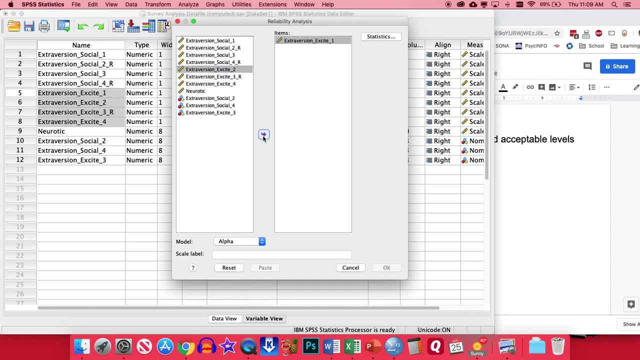 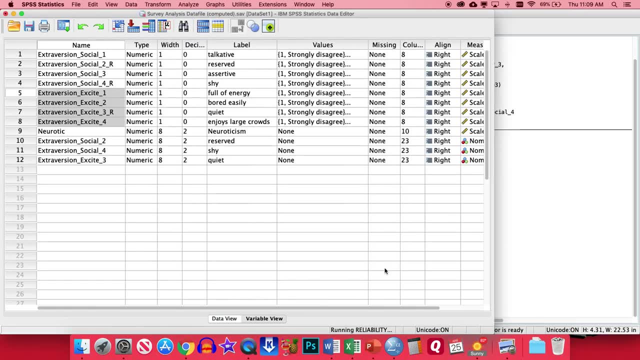 kick all of those and put in the excite items. So excite one, excite two, excite three and excite four. You notice I skipped the one that had an underscore R in it. So if I click, OK, I'm going to. 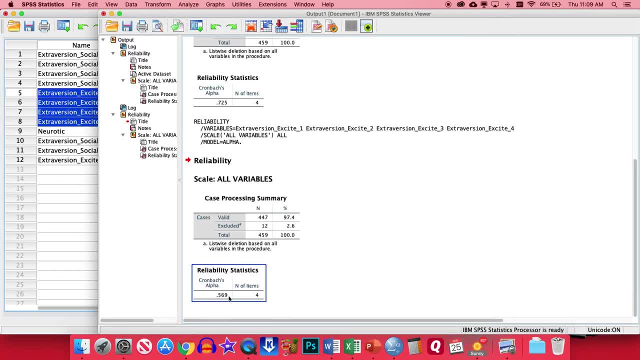 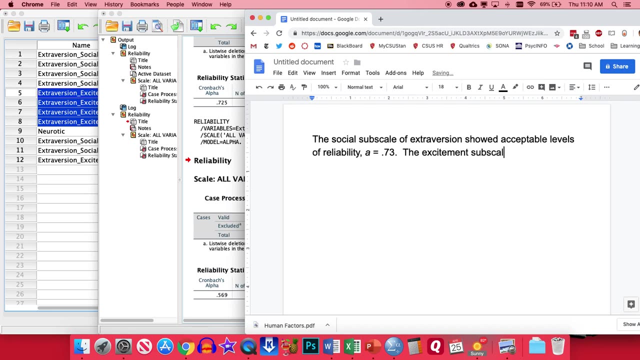 check out this result. This one actually showed less than acceptable levels of reliability. It had an alpha score below a 0.7.. In this case it was 0.569.. So in this case the write-up would be a little different. We'd say the excitement subscale of extraversion showed unacceptable. 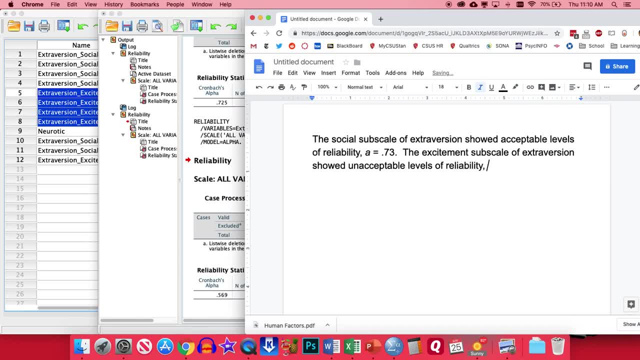 levels of reliability, And then once again we'll put in the lowercase a and this one round to a 0.57.. If the write-up either way is not that different, you're just saying whether or not it met that threshold of being a 0.7 or higher. If it did, it was an acceptable level of reliability, or? 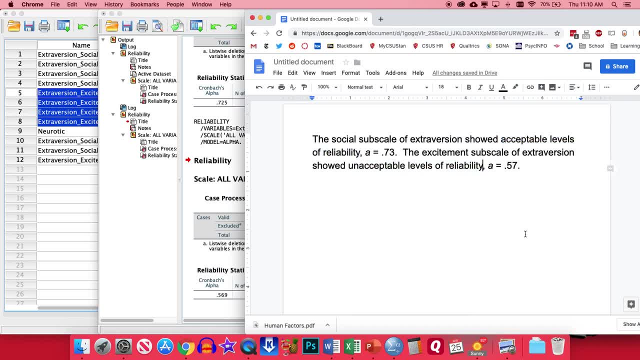 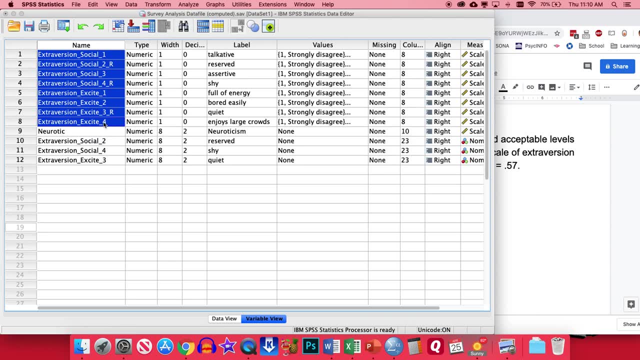 is reliable. If it didn't, it was an unacceptable level or it was unreliable. So, moving on from that, one thing we might want to test out is to see if these extraversion items correlate with something that we would expect them to. In this case, I have a measure of 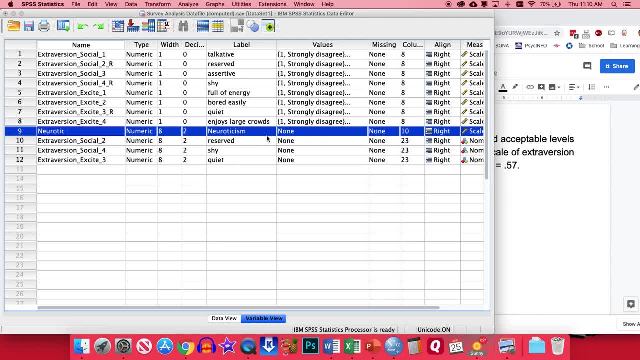 neuroticism right here, or it's an average of a neuroticism scale And typically if people are higher in extraversion they're going to have a higher level of reliability. So I'm going to see if they're lower in neuroticism. So we would expect a negative correlation there. Now to see. 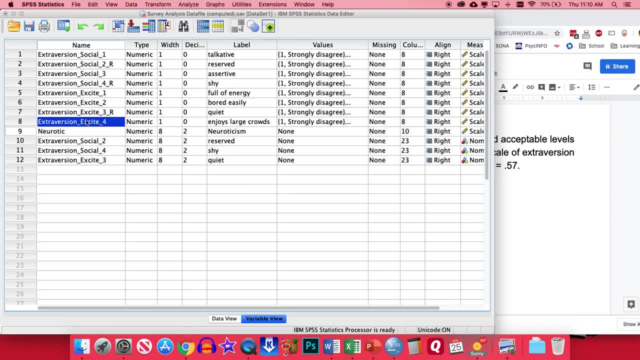 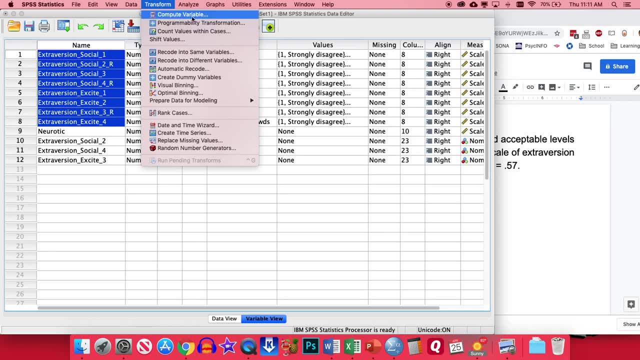 if that holds true, we need to also create one variable that is the average of all these extraversion items. So to do that, let's go ahead and create that. We're going to go transform compute variable, because we're going to be using some math here And for this one, basically, 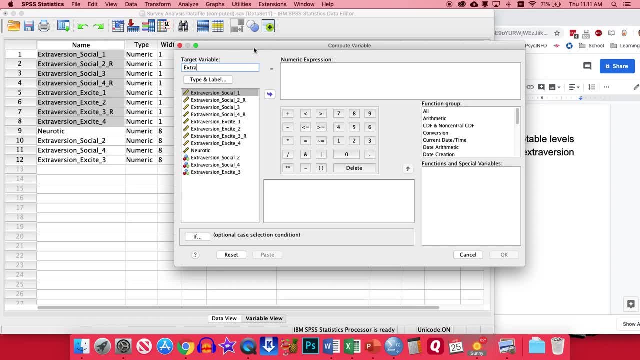 I'll create a variable called extraversion And this is going to be the average of all these items. So to average it, we can add them all together and divide by the total number. So putting them in parentheses first, the ones we're going to add in, we're going to add in item. 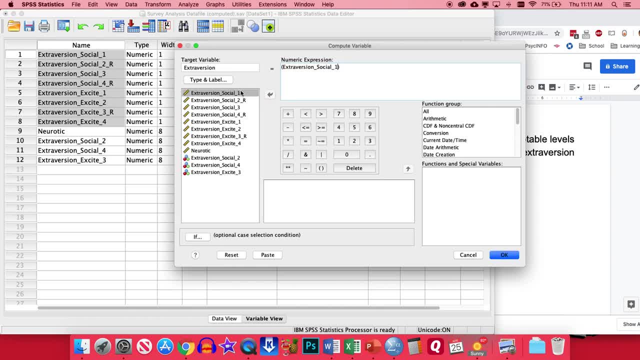 one, And it doesn't matter what order we put this in, but I'll keep it in order here. So item two are. we're going to skip over, but we're going to add the item two that we created. that's pointed in the correct direction, And so we're just going to add them all in. We're going to include all. 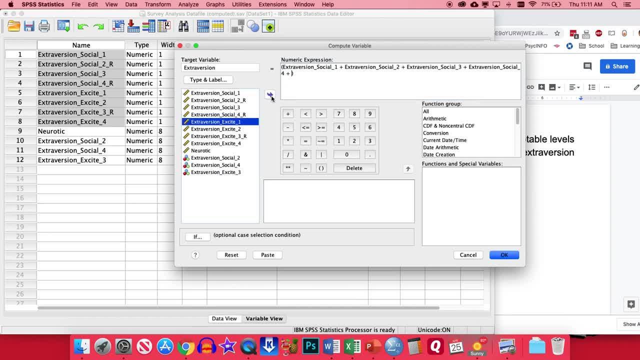 the items, this time from the social and excite subscales, because those are all part of extraversion And let's see, pop in, there we go. And so we want to see here is that we haven't missed any items. We have social one, two, three, four, excite one, two, three, four. And since we have 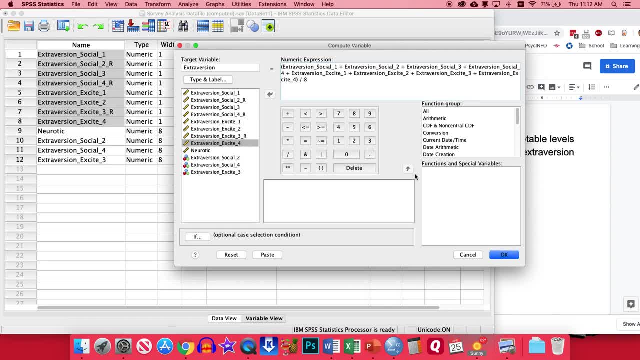 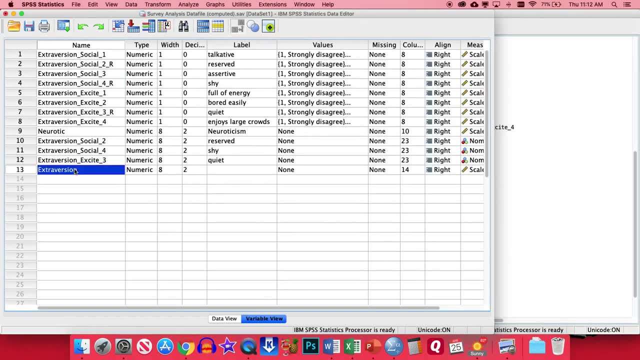 a total of eight items. we'll end by dividing by eight. So after you have all this, this is going to create our average. We'll click OK And it'll pop up at the bottom of our data set. I like to give this a label, So we'll call this extraversion, because the label end up showing up in our graphs. 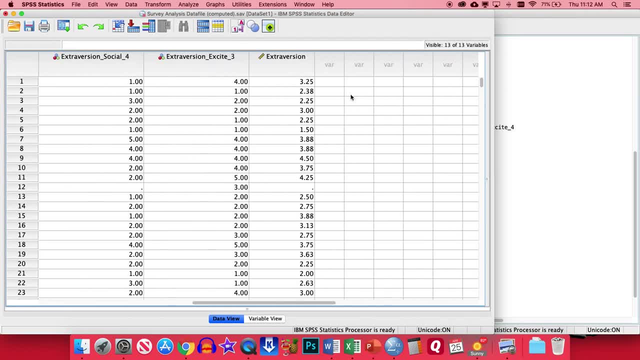 And if we go to data view, we should see that these are basically, you know, decimal places like 3.25,, 2.38.. And one thing you'll notice is that we don't have anything below one or above a five, because we're creating averages of one to five items. So, since they're all within that range, 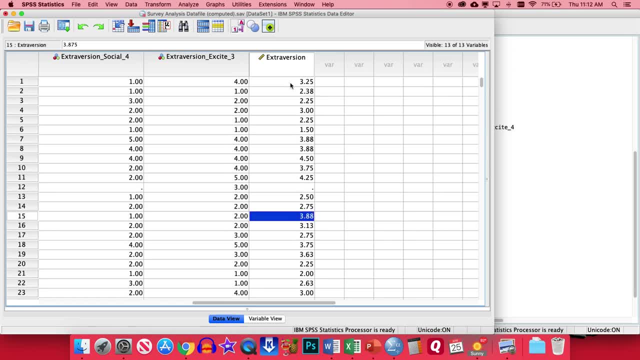 that means we probably did it correctly. If you notice a number that was below one or above a five, then we probably would have done something wrong. We'd have to redo it, But anyway, that looks good. So now we're going to go ahead and create our average, And we're going to go ahead and create 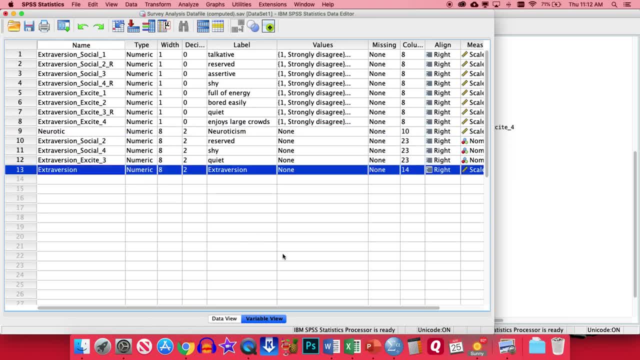 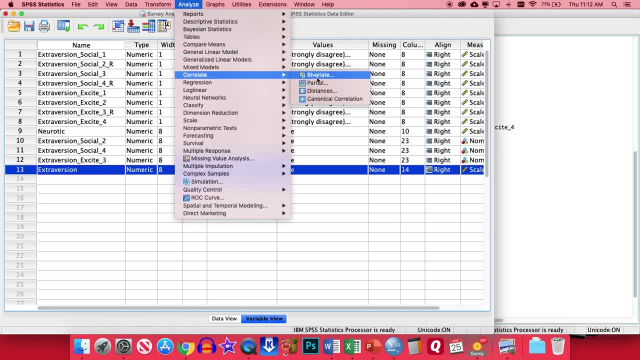 our average. So to test our final hypothesis that neuroticism and extraversion should be negatively correlated together, if we're doing a good job measuring extraversion, let's go to analyze correlate bivariate And we're just going to pop in our two items: extraversion and 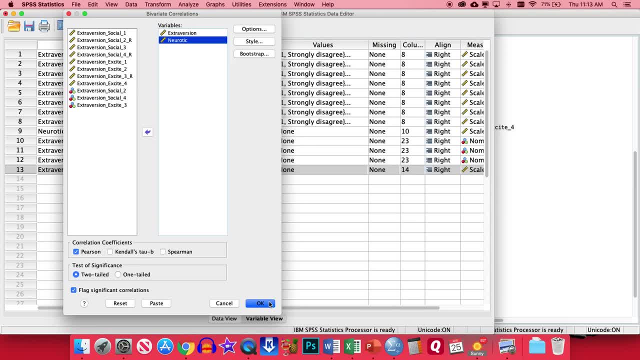 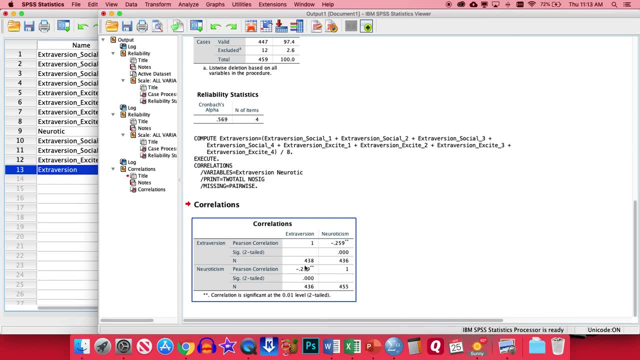 neurotic. We can just click OK with this. It'll tell us if they're correlated or not. And here, if we look right here, we're just going to pay attention to where neuroticism and extraversion meet in the table. So this set of three numbers right here. 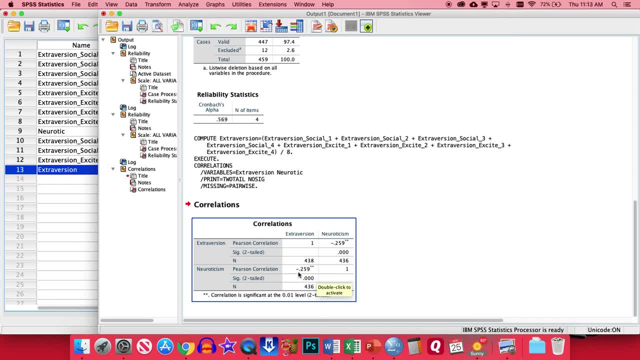 it looks like we do have a negative correlation. It's negative 0.259.. So a little bit on the weak side. It's around a 0.2 or 0.3.. But it is significant because right here it says sig. 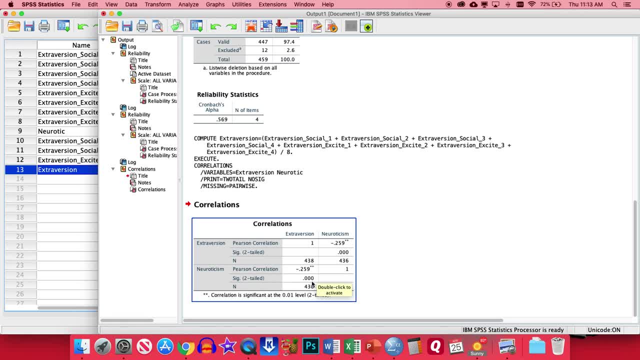 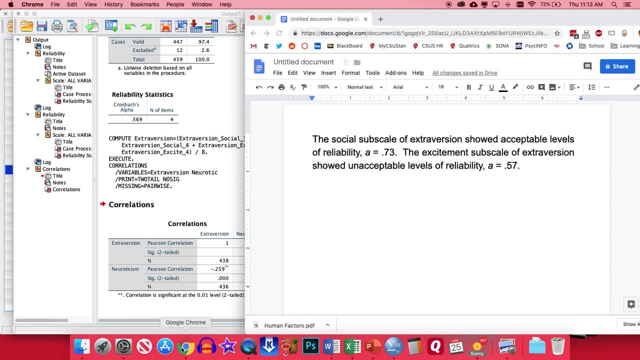 two-tailed, It is at or below a 0.05.. So it's definitely significant. So to write this part up, let me put this over here. We're basically going to say that it was found that extraversion was negatively correlated with neuroticism. 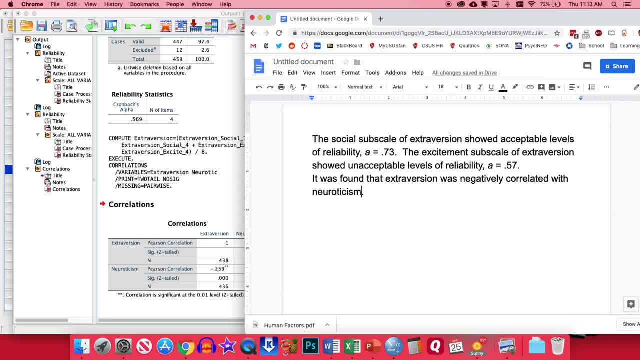 So I always like to write the result in plain English first, And then, basically, we're going to put in our R statistics And I'll just do some placeholders for right now. So the first thing we're going to do- I'm not quite sure what it did there. 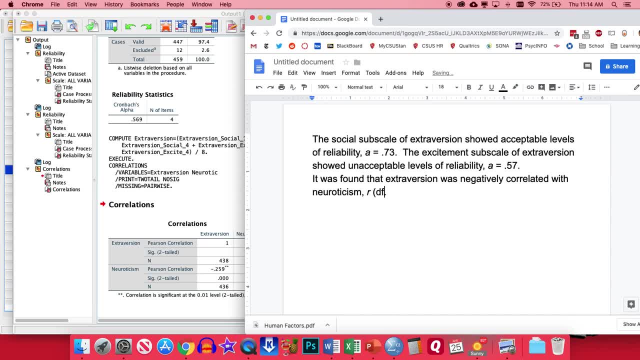 put in a lowercase r, Then we're going to do our degrees of freedom, And then the R value, followed by the P value. I'm already italicizing the parts that we need to italicize there. Now, the only thing it doesn't tell you outright is the degrees of freedom. 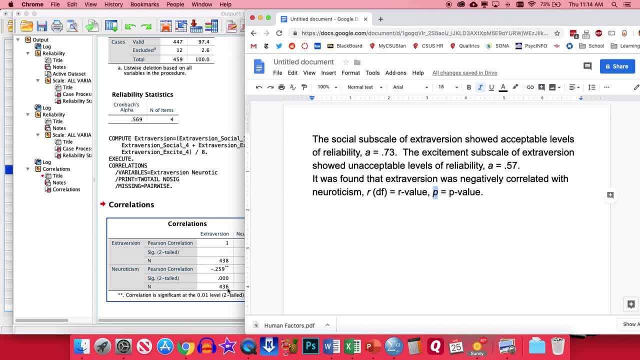 But for R, the degrees of freedom, is n minus 2.. So our n is 436.. So 436 minus 2 equals 434.. Our R value is what it's showing us right here, the Pearson correlation value, And it's negative. 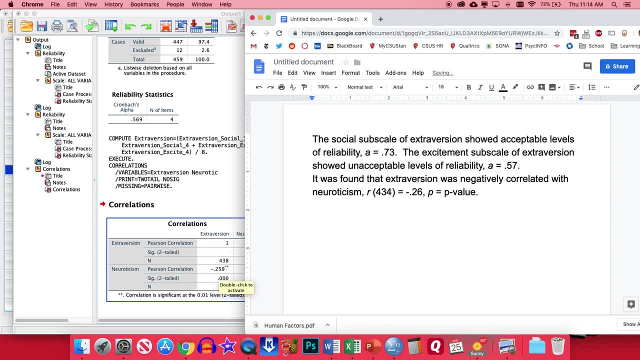 0.26.. We round that to the 100th place. And then finally, for the P value. it's so low we can't actually report it. For example, we couldn't write equals 0.00.. That's. 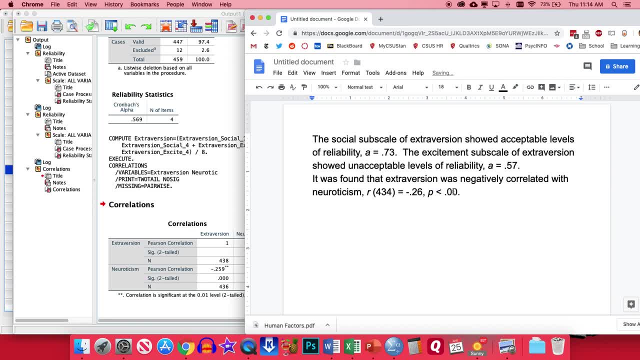 too low, So we change it instead- is less than 0.01, because that's as low as we can report it in APA formatting. So basically, this confirmed hypothesis: we're probably measuring extroversion pretty well because, as expected, it's negatively correlated with neuroticism. 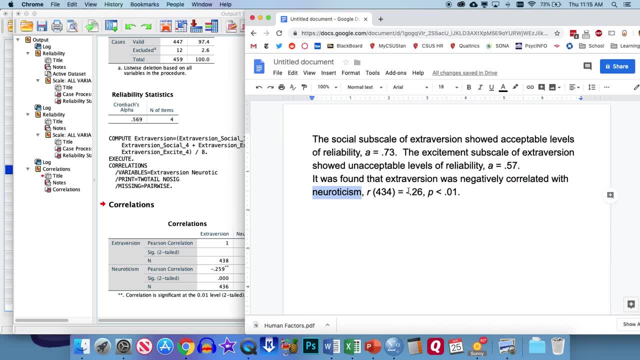 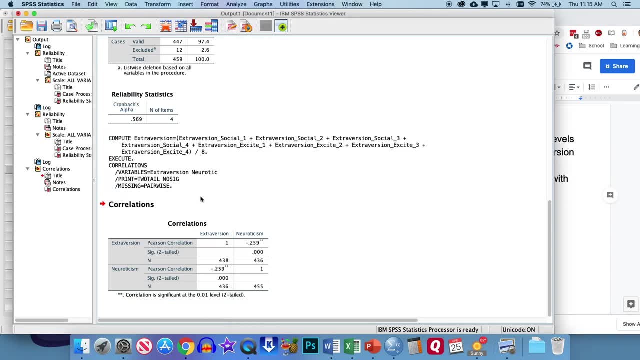 which is basically how depressed or anxious people are. We'd expect if people are highly sociable, they're probably less depressed. Now, the last thing, since this is a very correlation. we can create a graph for this, a scatterplot, So let's go to graphs. legacy. 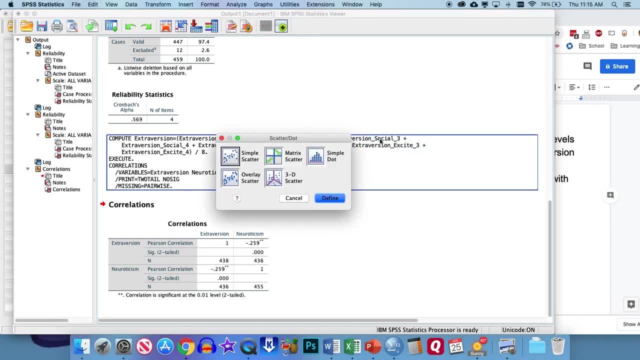 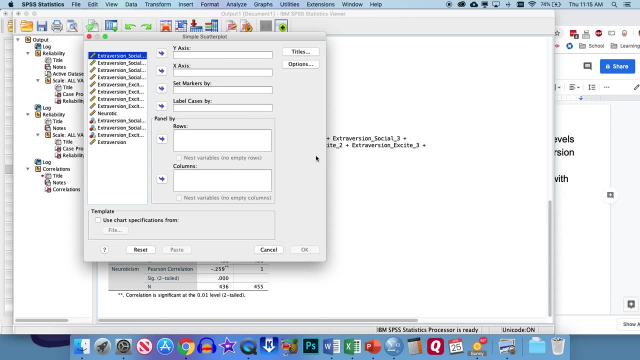 dialogues, scatter, slash, dot, And we're going to keep it at simple scatter, click, define, And we're just going to pop one of our variables into the y-axis and one of the x-axis. It really doesn't matter which one we put in which axis. I'll just put neurotic in the y-axis and extroversion. 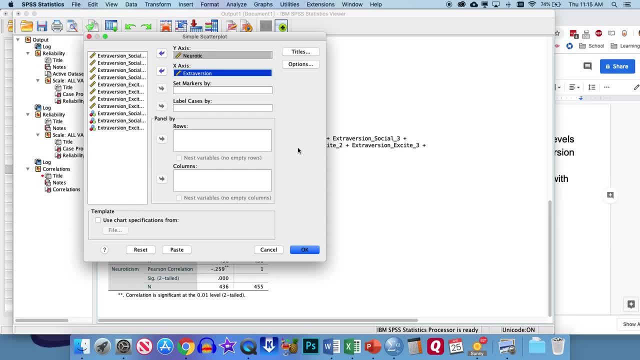 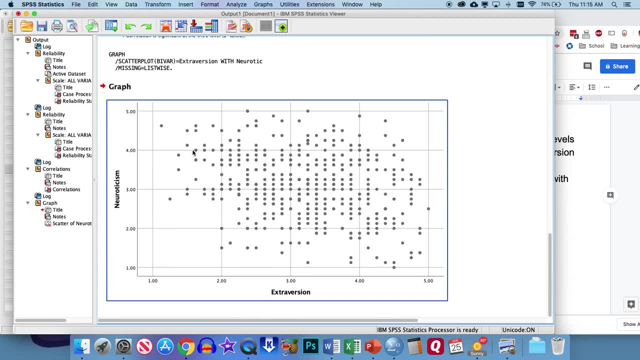 in the x-axis, But you can easily flip those. It'd be the same result. So if we click OK, it'll generate our scatterplot graph here, As you can tell. you can kind of tell it's a little bit of a negative skew. 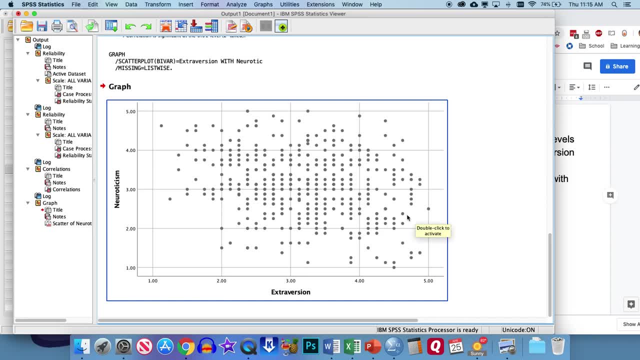 but it's kind of hard to read exactly where the best fitting line would be. So let's go ahead and add that regression line to really show the relationship between neuroticism and extroversion. To do that, we're going to double click to go into chart editor And then, once that pops up, 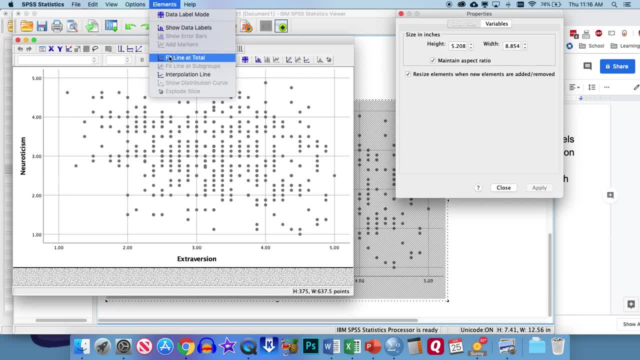 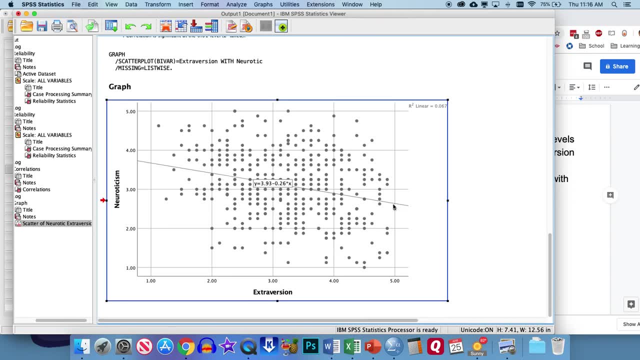 go up to elements and click fit line at total. That'll put the regression line on there. We close this. it goes back to original graph And there you can really see that there is a negative trend there. The high-end regression line is the one that's going to be the most. 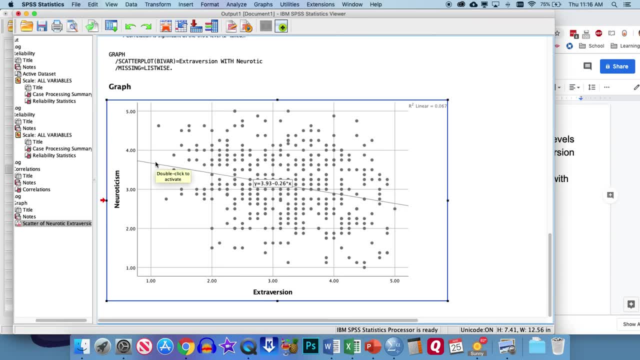 visible and how high your people are in extroversion, the lower they are in neuroticism, and vice versa. So we're just going to copy this. We'll go copy as image Or if you're on windows, you go copy special and then select image And then we always are going to put this on a separate.